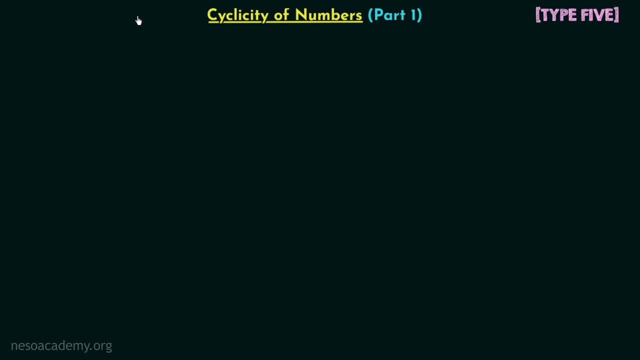 So the first question is: what do we mean by the cyclicity of a number? The cyclicity refers to the repeating pattern of the unit digits of the powers of a number. So when we have a number and we start increasing the powers of that number, we will find there is a repeating pattern of the unit place, or 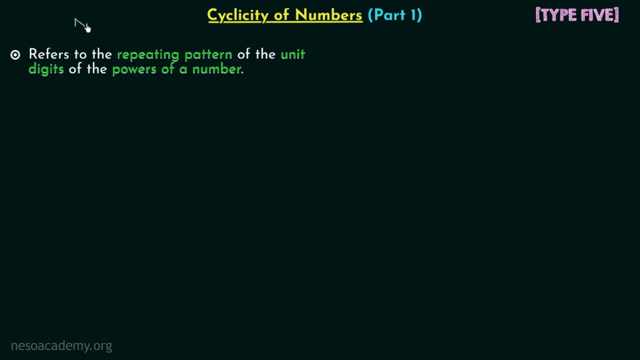 unit digits. For example, let's say we have a number n and the power of that number is n. This number is small, n. Now when we start increasing the power n, we will find the results will have a repeating pattern of the unit digits. or we can say the unit digits will. 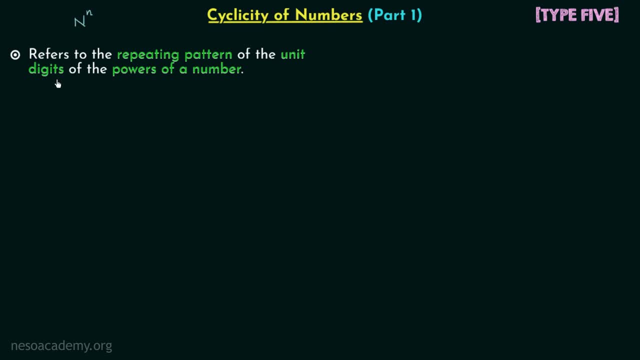 follow a predictable cycle. So there will be a cycle at the unit place of various powers of a number and this we call as cyclicity of a number. So I hope you understand what do we mean by the cyclicity of a number, and this concept will become more clear when we will solve some examples. 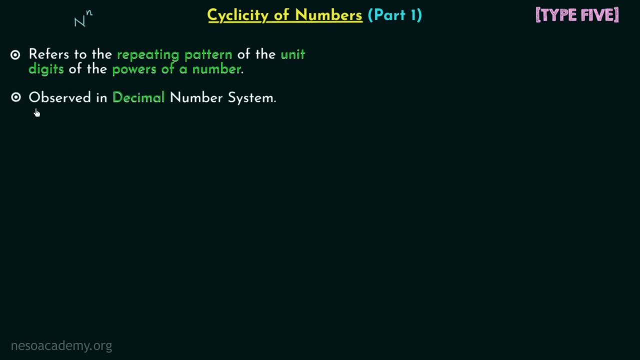 Now we will move on to the next point. Cyclicity is observed in decimal number system, So the repeating pattern or the cycle we just understood, will be found in decimal number system and therefore we will find the cyclicities of the decimal digits only And the cyclicity of a 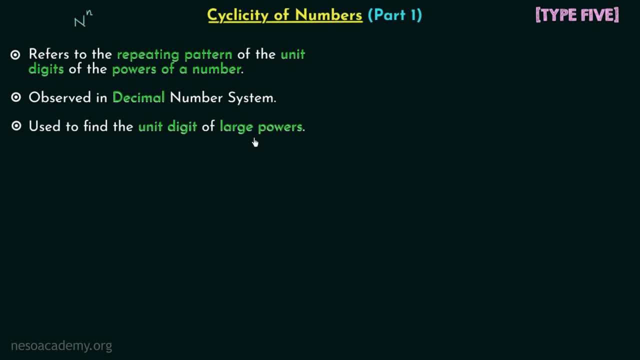 number can be used to find the unit digit of large numbers. So let's move on to the next point. So when the value of n is large and we are interested in finding out the digit at unit's place, then we can use the knowledge of cyclicity to find out the digit at unit's place without 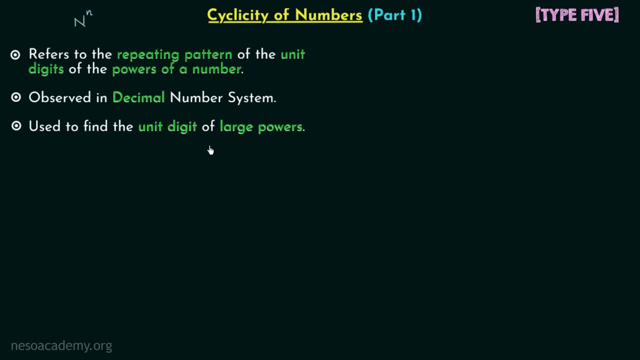 going through tedious calculations. So we use cyclicity to find the digit at unit's place when we have large powers. So I hope all the three points are now clear to you, And now we will move on to our cyclicity table. The first column is having the digits of decimal number system from 0 to 9, and the second column 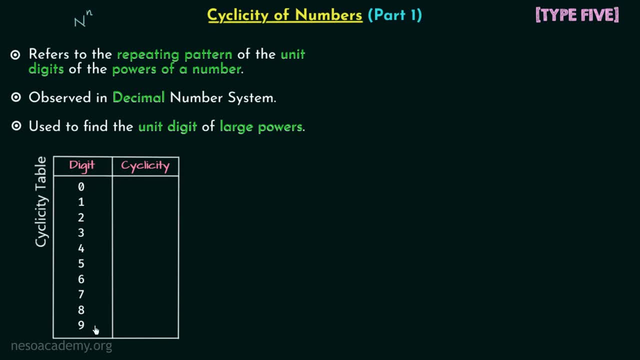 will have the cyclicity of all these digits. We will, one by one, find out the cyclicity for all the digits we have, and then, in the upcoming lectures, we will use the complete cyclicity table to solve the questions. So let's move on to our first digit, which is 0.. 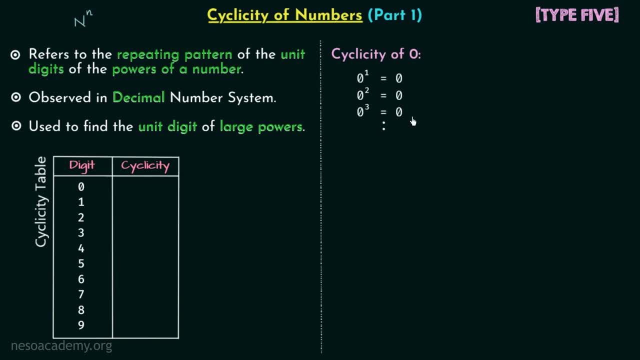 Cyclicity is observed in decimal number system from 0 to 9, and the second column will have the cyclicity of: 0 is 0.. To find the cyclicity of a digit, we will calculate the various powers of that digit and then we will analyze the different results which we get. 0 power 1 is 0,. 0 power 2. 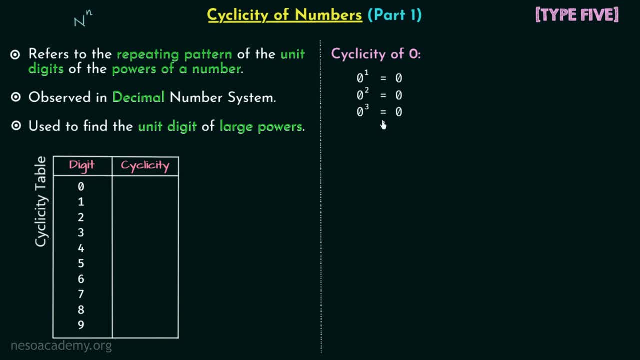 is 0, 0, power 3 is 0, and so on. So we are getting 0 every time, and this clearly means 0 will have the cyclicity equal to 0.. Now we will move on to the cyclicity of 1.. Like 0, in case of 1 as well, we are getting the same. 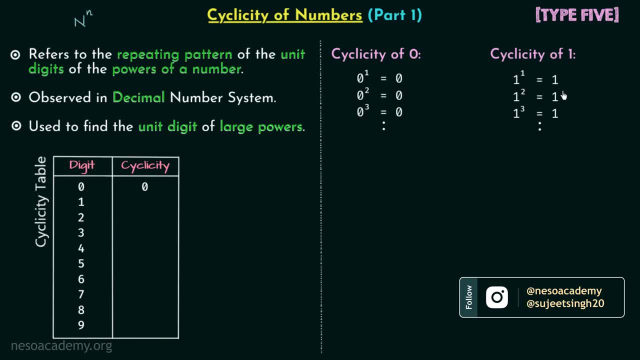 result throughout: 1. power 1 is 1, 1, power 2 is 1, 1 power 3 is 1, and so on. So 1 will have cyclicity equal to 1.. And now we will calculate the cyclicity of 2.. Like the previous two cases, 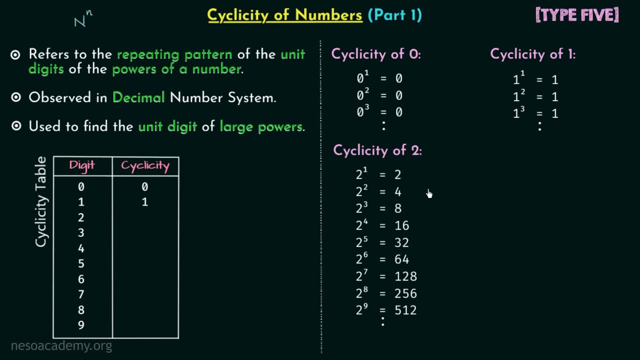 we have calculated the various powers of 2, but this time we will use the cyclicity of 1.. To find out the cyclicity of 2, we had to calculate the powers till 9.. We want a repeated pattern and to get that repeated pattern we had to calculate till 2, power 9.. Let's quickly observe the results. 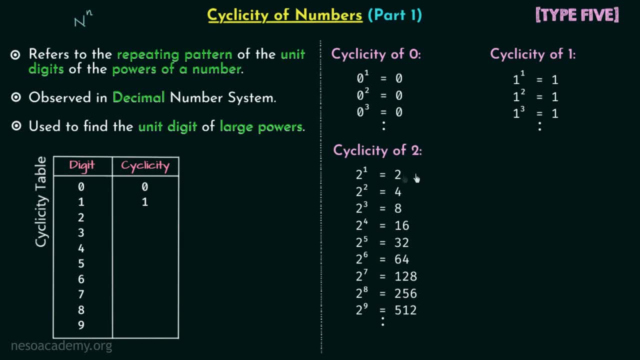 we have Focus on the unit places only. We want to spot the point from where we start getting the same unit digit. So let us start. We have 2, then we have 4, then we have 8, then we have 6.. Now, after 6, we are again getting 2.. We got 2 initially. Now, after 6, we are again. 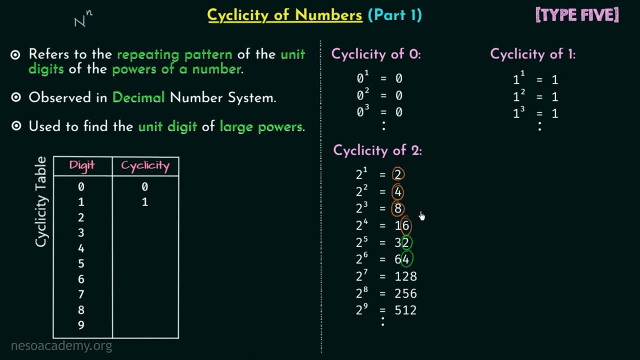 getting 2.. Then we are again getting 4.. Again we are getting 8.. Then again we are getting 6, and then again we are getting 2.. So this means the cyclicity of 2 is 2, 4, 8, 6.. You can see, we are. 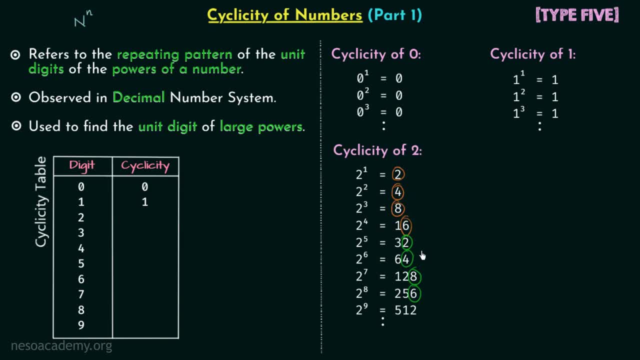 getting 2, 4, 8, 6, and then again we are getting 2, 4, 8, 6.. Similarly, we will get 2, 4, 8, 6 after this as well. So we have 2, 4, 8, 6 as the cyclicity of 2 and the. 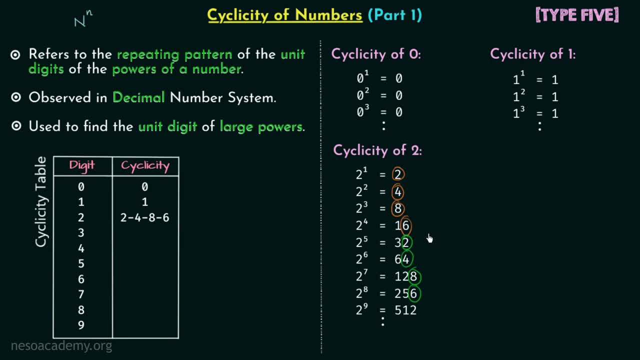 interval after which the repetition is taking place is equal to 4.. So this means the repetition is happening after the interval equal to 4.. And now we will move on to the cyclicity of digit 3.. Again, we have calculated various powers of number 3 to find: 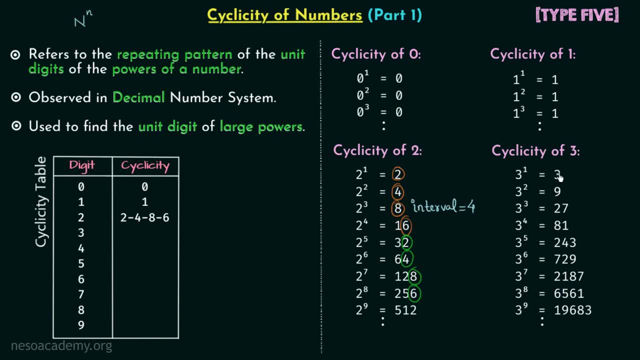 out the repeated pattern. Focus on the unit places of the results. we have 3- is what we are getting from 3 power 1 at the unit's place. Then we have 9, then we have 7, then we have 1 and then again. 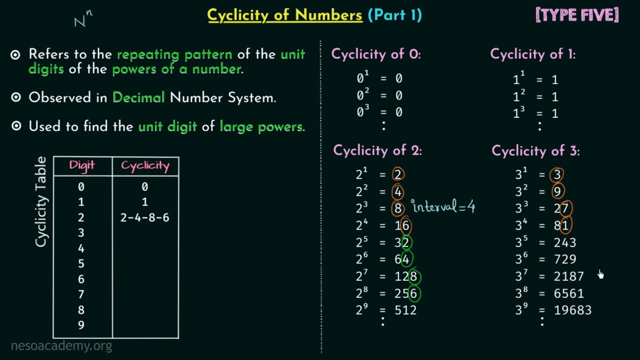 we are getting 3.. So this time we are going to get the cyclicity as 3, 9, 7, 1.. When you calculate further, you will again get 3, 9, 7, 1.. So this means we are getting 3, 9, 7, 1.. So this means 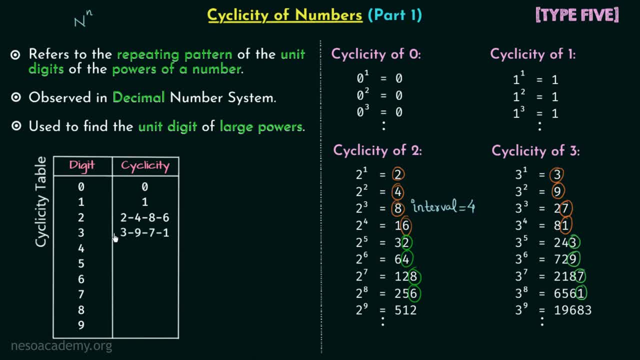 the cyclicity of digit 3 is 3,, 9,, 7,, 1, and again the interval after which the repetition is happening is equal to 4.. So you can see that the cyclicity of 0 and the cyclicity of 1 is kind of similar- See here in the table also, and 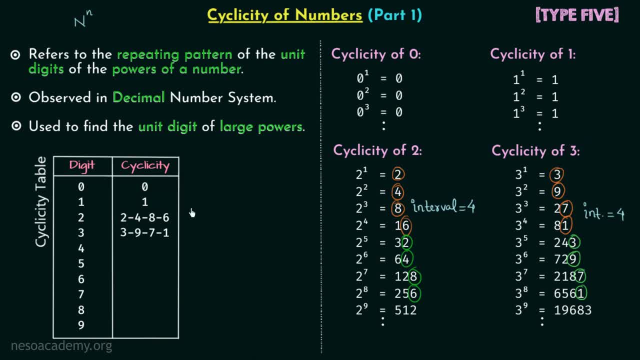 the cyclicity of 2 and the cyclicity of 3 is also kind of similar. For 2 we have 2, 4, 8, 6, and for 3 we have 3,, 9,, 7, 1.. Now consider this: So you get 2, 4,, 8, 6 and 3, 9,, 7, 1, and then again we have 9, 7, 1,. 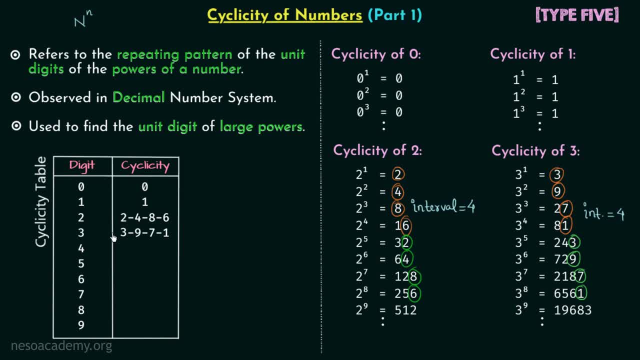 1.. So, like we saw in the definition, the digits at unit place are providing a repeating pattern for the increasing powers of a number. Now, moving on to the cyclicity of 4, I believe you can calculate the cyclicity of 4 on your own. Try to find out the cyclicity of 4 and